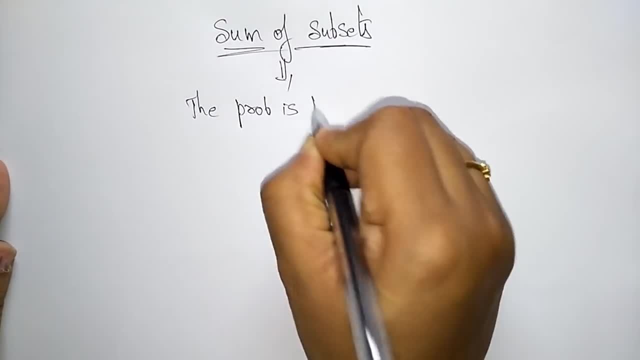 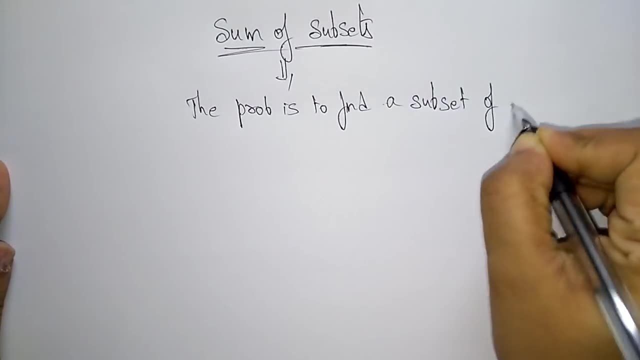 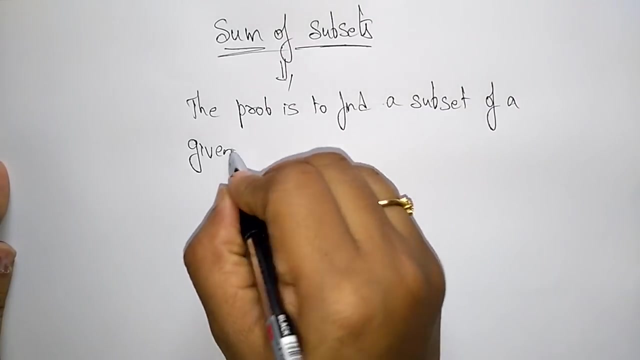 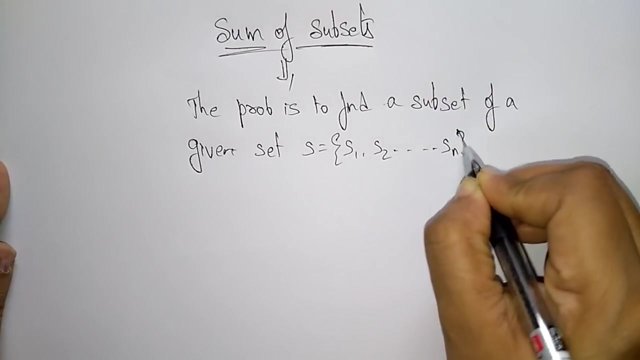 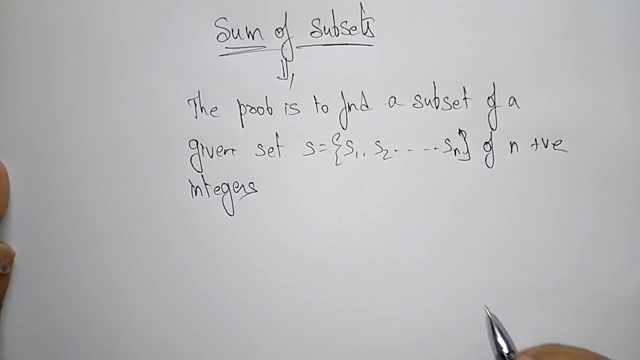 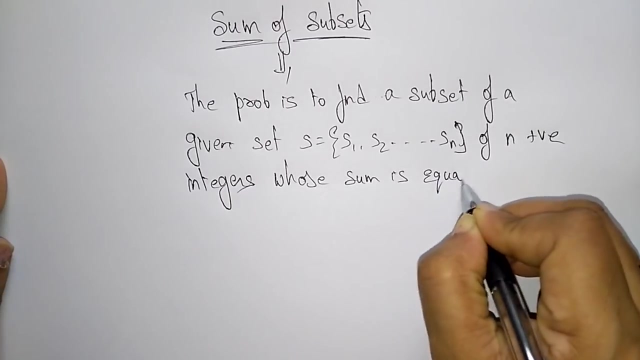 let me write the definition. The problem is to find a subset of a given set. We have to find a problem. The problem is to find a subset of a given set- S is equal to S1, S2 up to Sn- of N positive integers, N positive integers whose sum, whose sum is equal to. 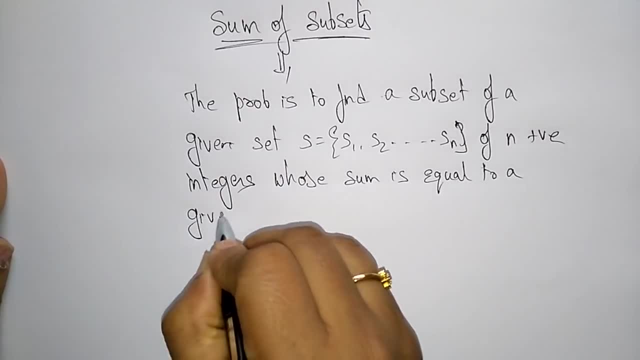 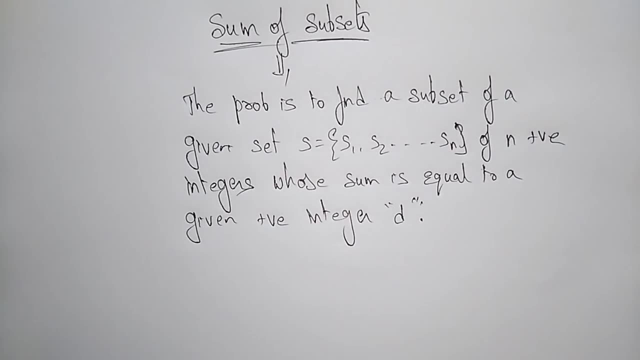 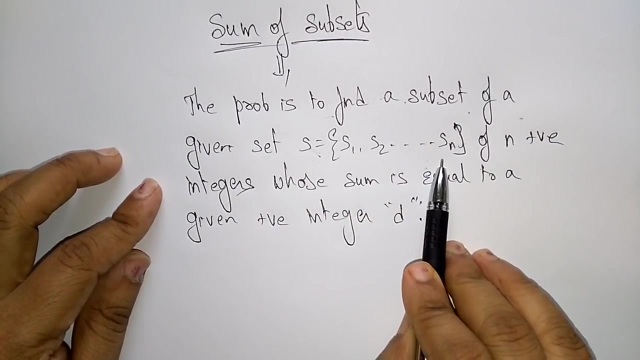 a given set, N positive integer D. So this is the definition of sum of subsets. So the problem is to find a subset of given set. So for this given set, S1 to up to Sn, for this given set, we have to find the problems for subsets. 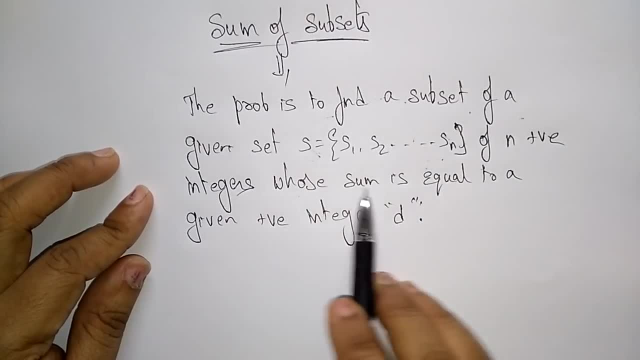 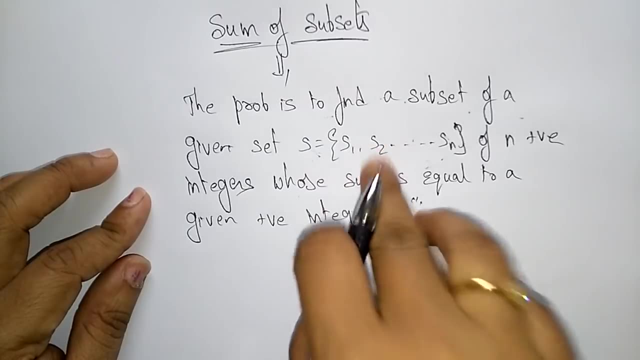 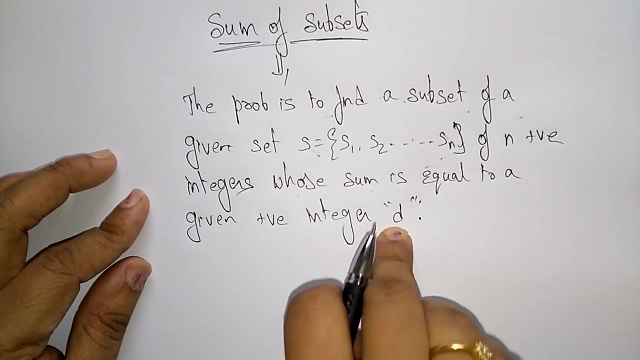 different subsets are there of N positive integers whose sum is equal to given positive integer N. So whatever the subset that we are finding out from this set, that subset should be equal to the sum of the equal to the given integer. that is a D. 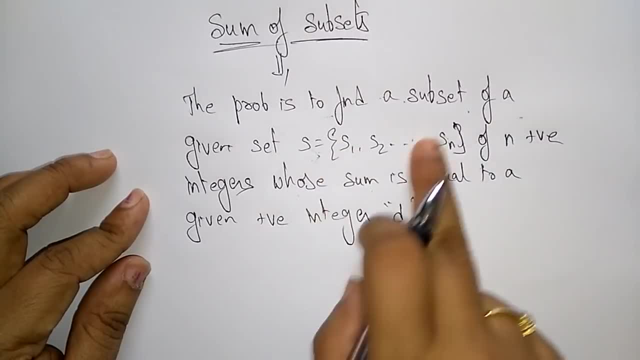 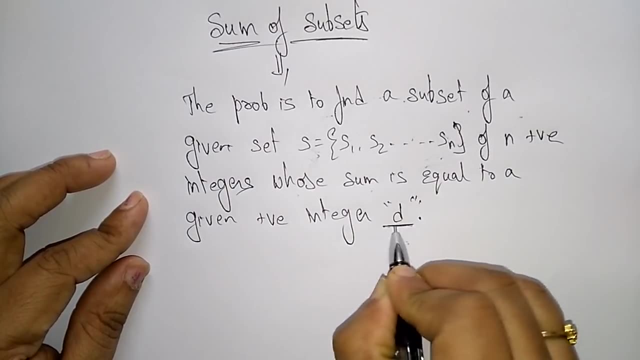 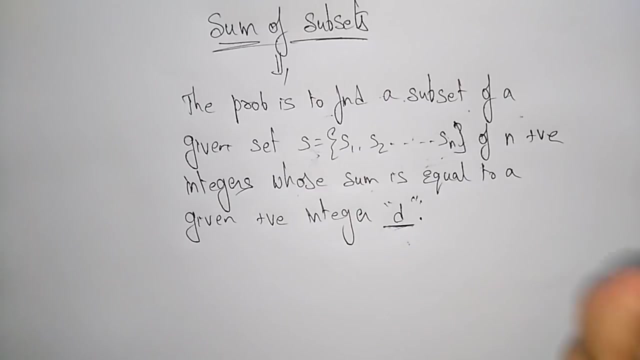 That should be equal to that sum. So, whatever the in this set we have to find out some integers. Those integers should be equal to this integer, sum of this integer. So sum is equal to a given positive integer, that is a, D, So that is a condition for sum of subsets. So just, we have to. 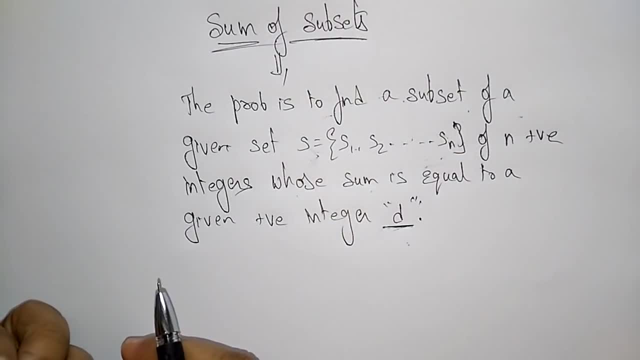 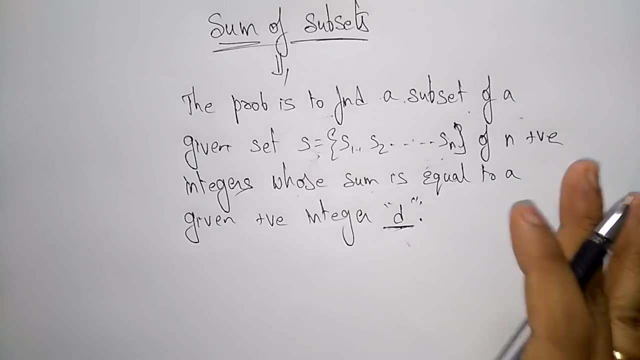 in this set that we have to solve those subsets and finally we have to find out this integer. So here the observation is: it is convenient to sort the set elements in increasing order. So let us take whatever the problem we are given, So that in that problem we have to make 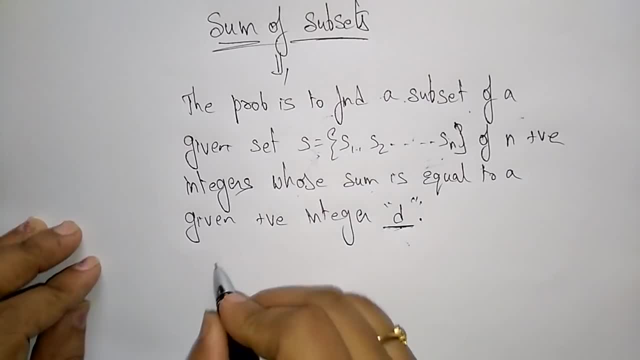 arrange the elements that should be in increasing order. That is, S1 is less than or equal to S2 is less than or equal to up to S. less than or equal to Sn. So that is, we have to solve those subsets. So that is, we have to solve those subsets. 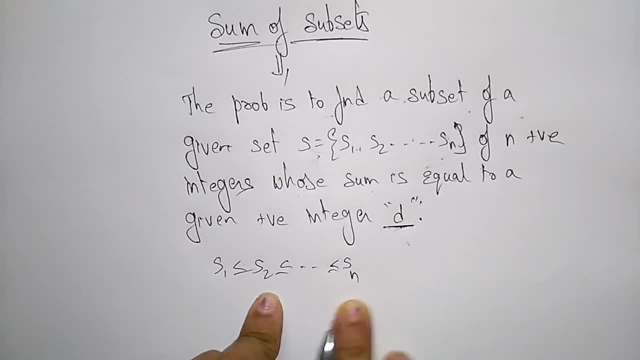 increasing order and each set of solutions don't need to be necessarily a fixed size. and one more condition is: whatever the you are finding out, the set of solutions for the given problem, there is no need to be necessary. that should be a fixed size. now let us take one. 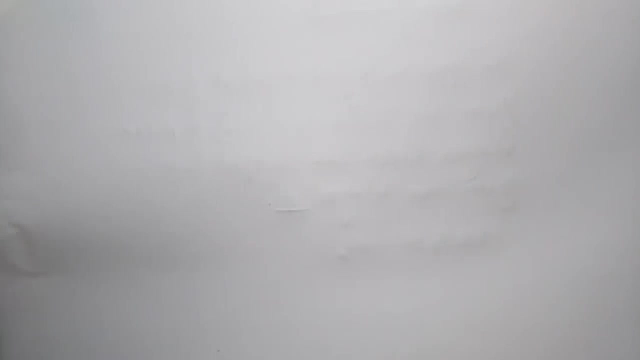 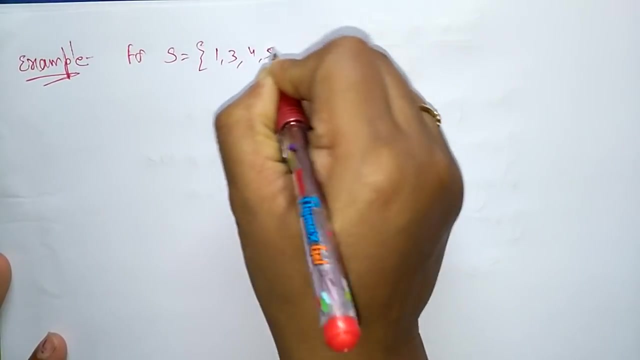 example for the sum of subset. let me take the example. so here is an example for finding out the sum of subsets. let us take for set s is equal to the set consisting of four elements: 1,, 3,, 4,, 5 and the. in this set we have to select a subset so that subset should be: 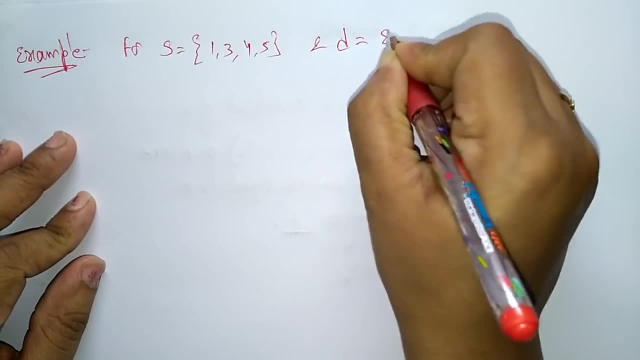 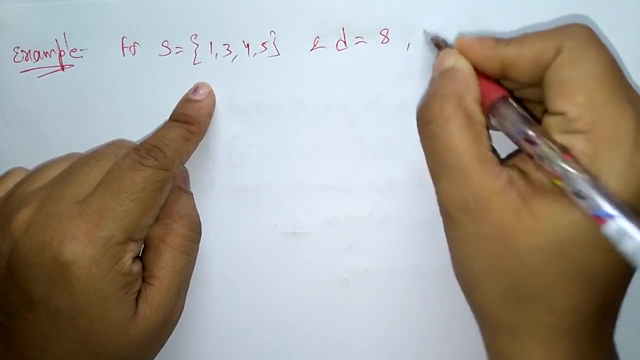 equal to that number. the integer number is 8. the total should be 8. okay, so from this set, what is the total that should be 8? what are the sets that can subsets that consists of? the total is 8. so from this set we have to select a subset that is 8. so from this set, we have to select a. 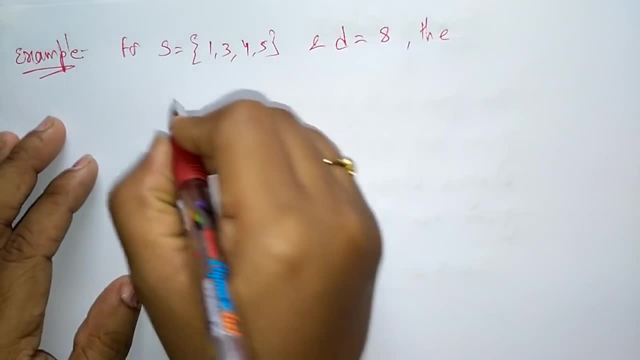 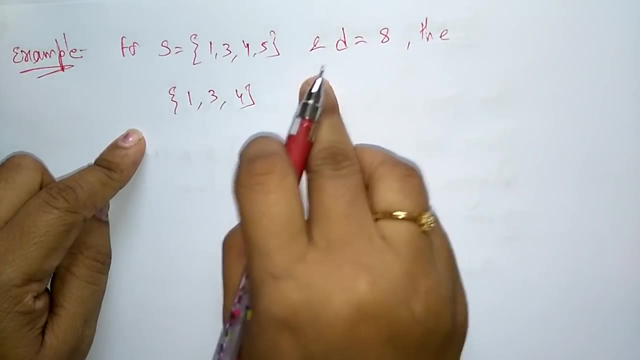 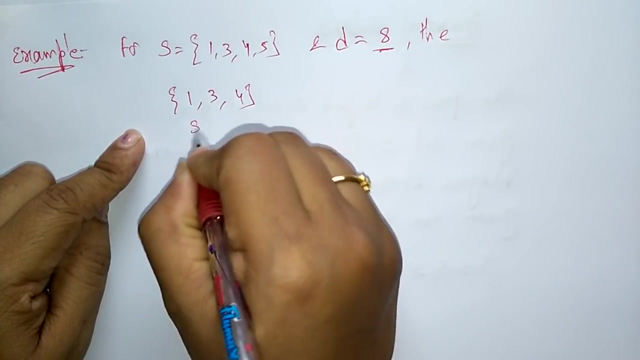 is 8. and one thing: the number should be an increasing order. suppose, if i take 1 comma 3 comma 4, what is the total? 1 plus 3, 4, 4 plus 4, 8. okay, i got, i got the solution. i got the integer. so this is solution 1. so is there any say? so subsets that the result is equal. 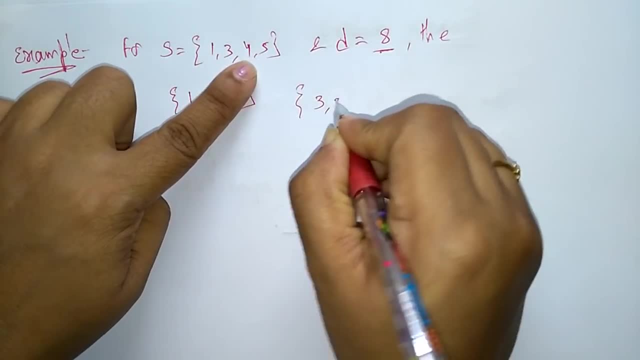 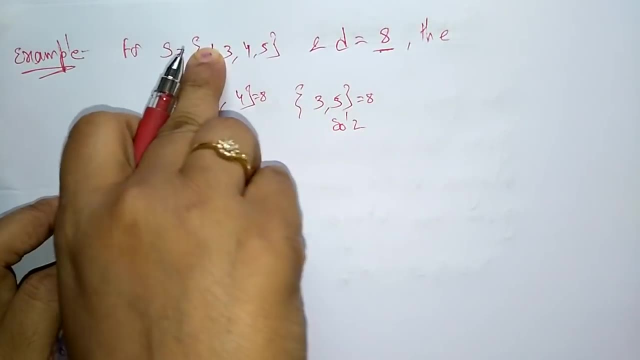 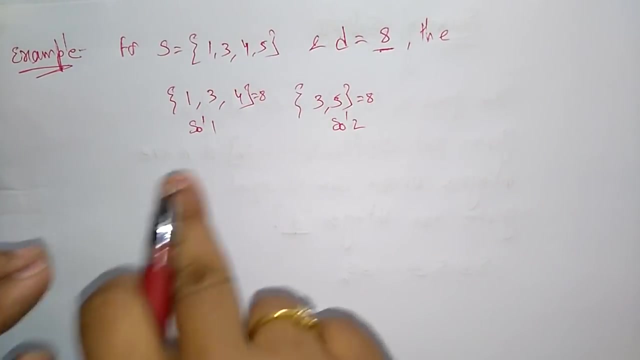 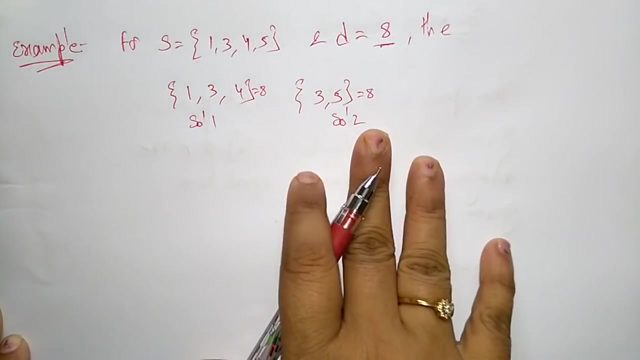 to 8 or 3, 5, so the solution, the answer is 8. okay, this is another solution. so from the given set there is more uh. i got uh, two possible solutions. so number of uh. i'm having two possible solutions for the given subset. so this is a subset, sum of subsets we call it is. so let me explain. 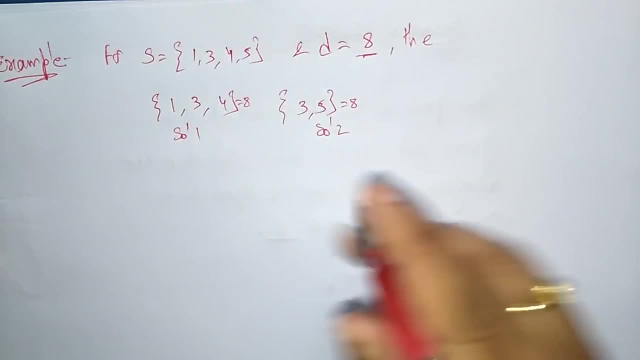 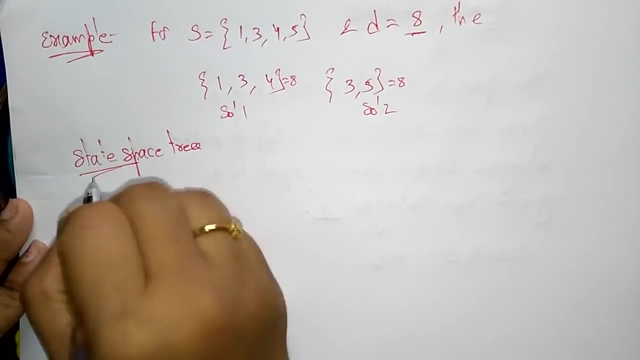 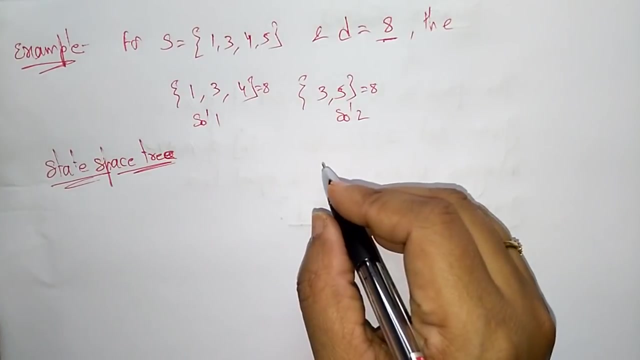 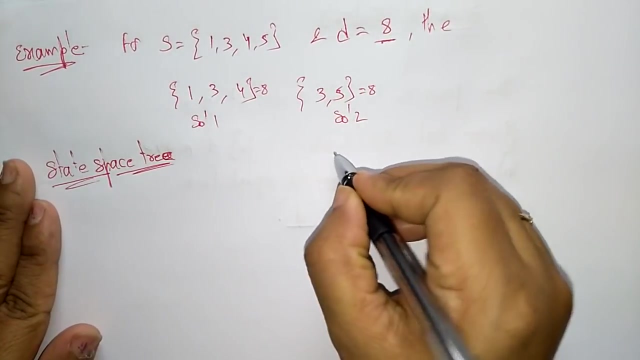 uh, this problem by using the state space tree. let me draw the state space tree. how you, how we are going to calculate this problem by using state space tree. so before starting the state space tree, there are no elements are inserted. so if no elements are inserted, the it should be start with. 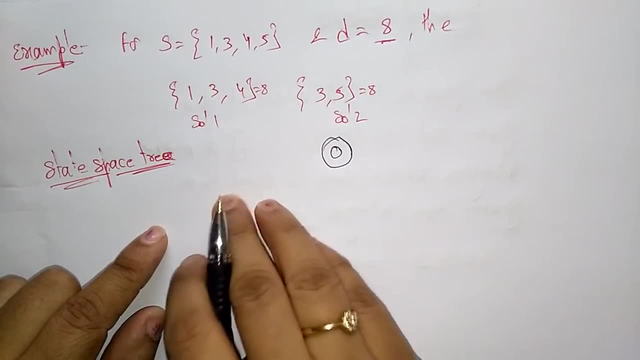 zero. okay, so the starting node should be zero, because if there are no elements are inserted, the it should be start with zero. so if there are no elements- areIONまあ elements in a tree- first start with zero. so the first element that should be inserted is: 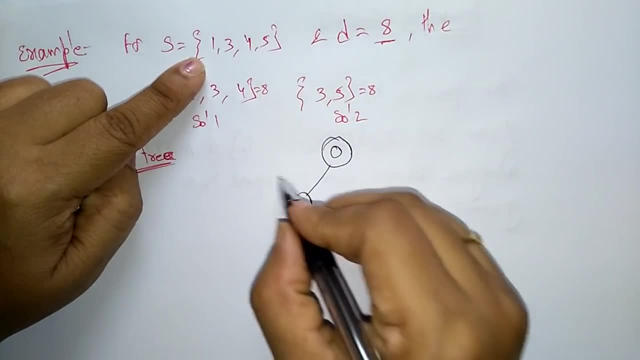 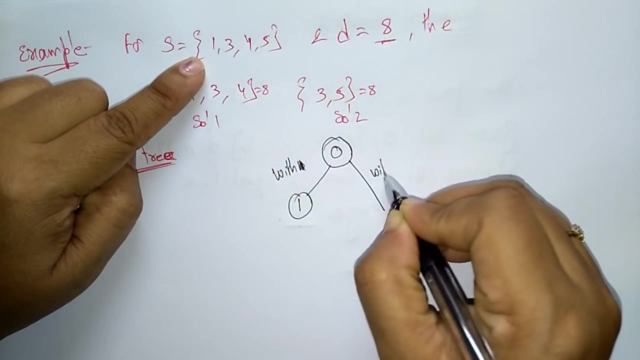 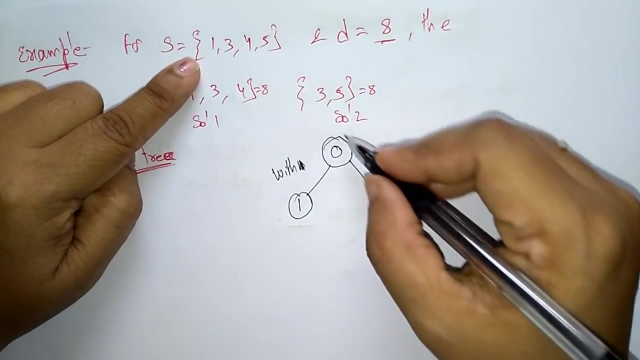 one. so what are the subset of these zeros? so they should be with one, with one and without one. so without one means just copy the zero. left side, just right side, just copy the zero and right side, just add the first element. that is a one. so now next coming. 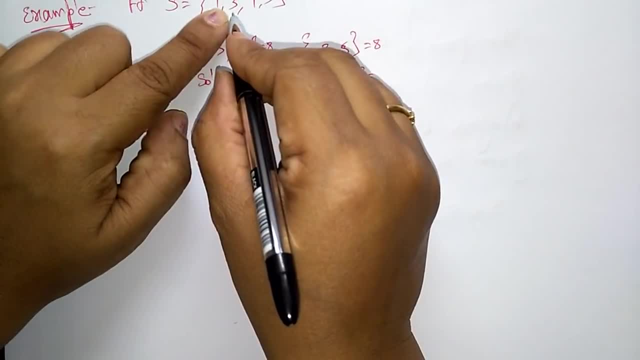 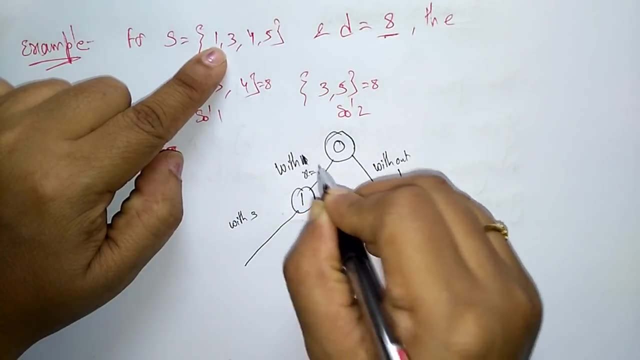 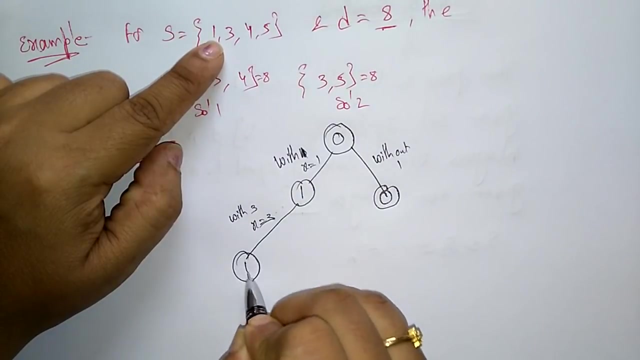 to that. so the next element is three. so what is the solution with? with three means you could here: x is equal to one, x is equal to three. so with the three, three plus one, you will get four. the subsets for this one is with three and without three. without three means just copy. 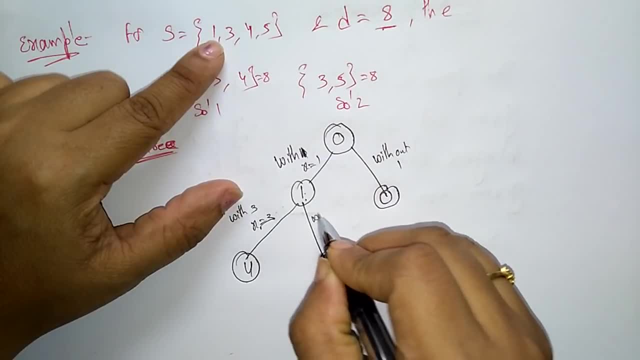 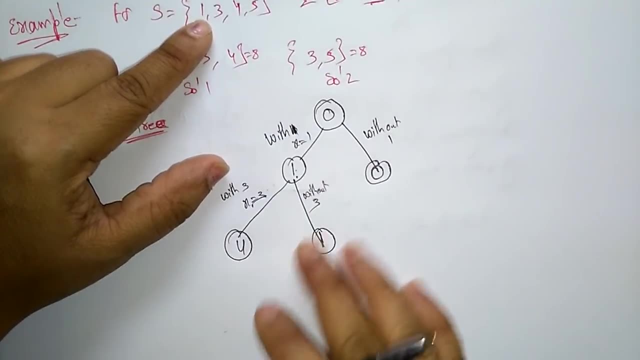 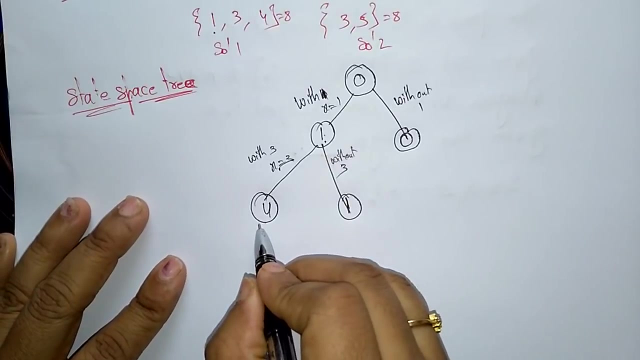 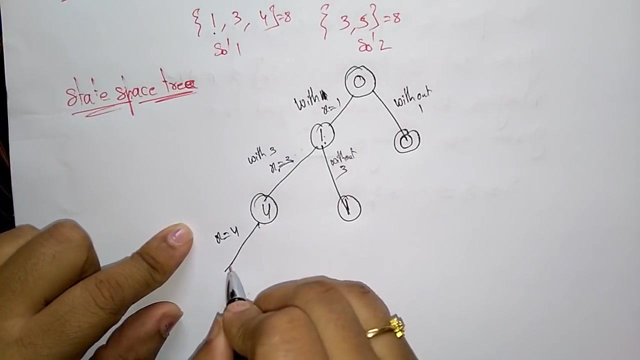 one, just copy one without. without. three means x is equal to three. x is not equal to three. that's it. so again. next coming to this next element is four. so you have to add four. x is equal to four, means with four, four plus four, i'll get eight as an answer. so eight, which is 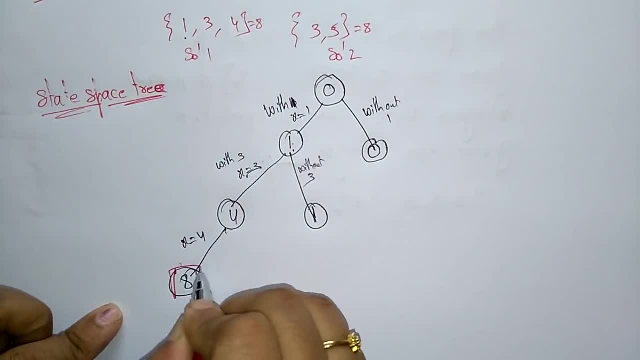 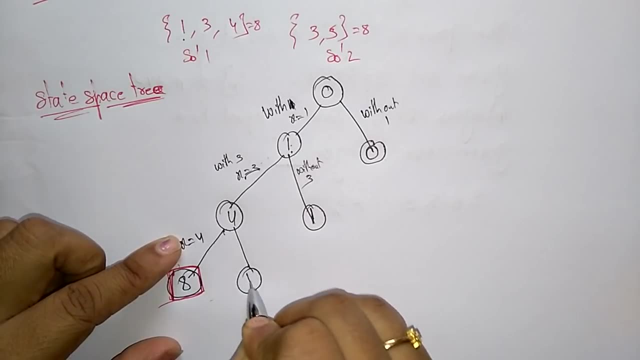 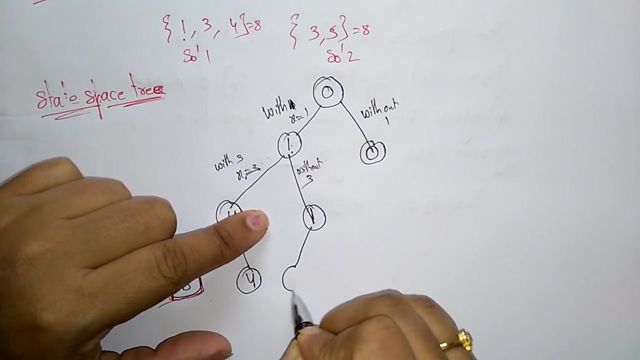 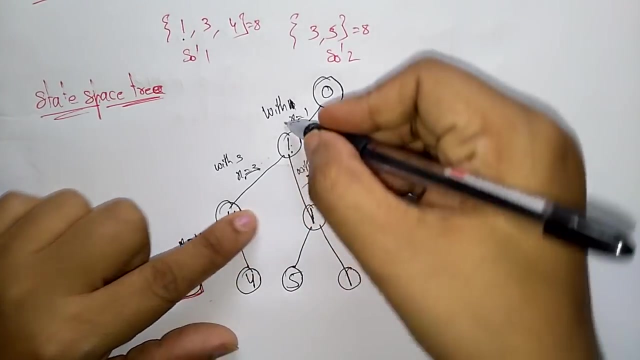 the element, which is that i have to get. so this is a solution, the first solution i call. so with four and without four, okay, and for this with the four, okay, four plus one, five without four, just copy this element, one, okay. so, right side, just copy whatever the element that is there in the tree, that root node consisting of: 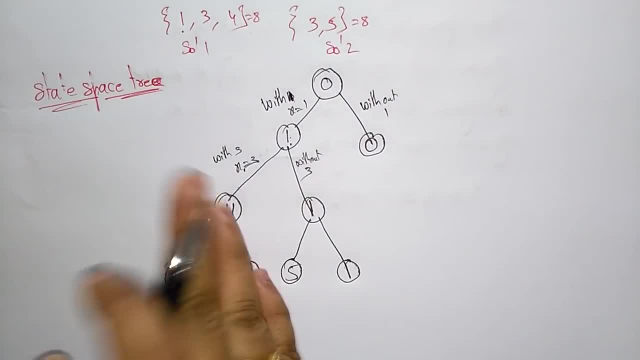 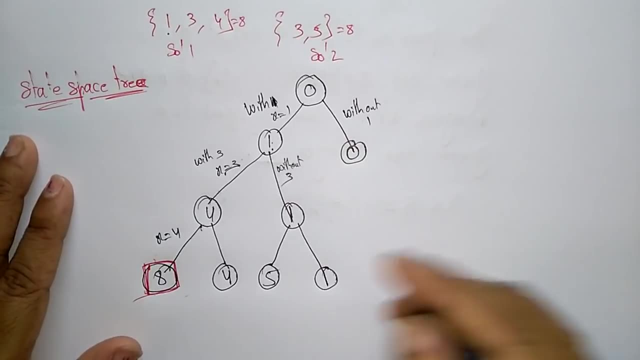 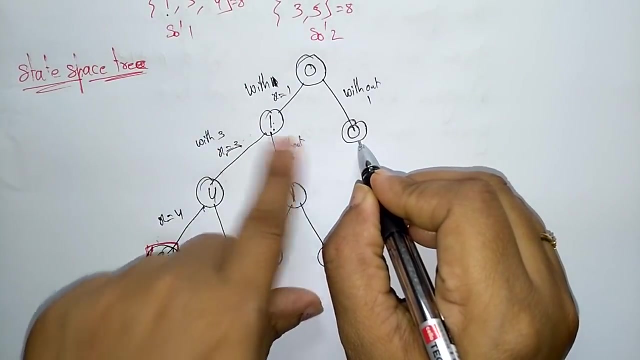 node consisting of means, this is with node and without node. this subset consisting of with and without, with with element and without element, those two elements will be present in that set, the phi 1. and now coming to here, so this is with with 3, we are calculating, so with 3. 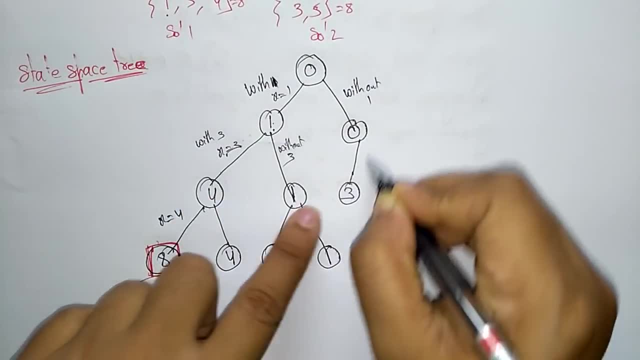 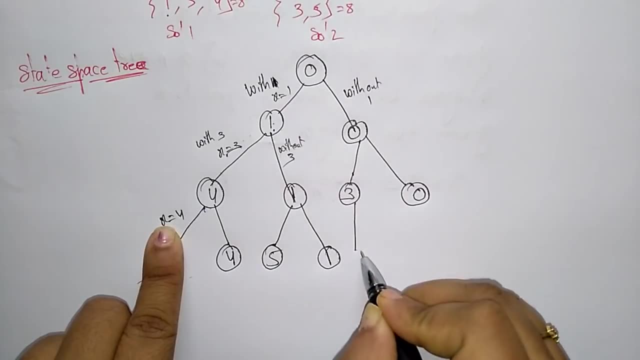 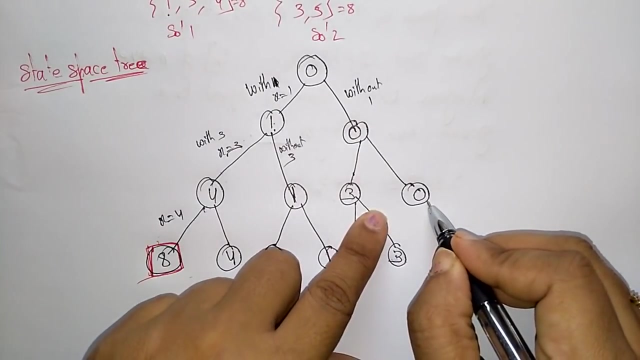 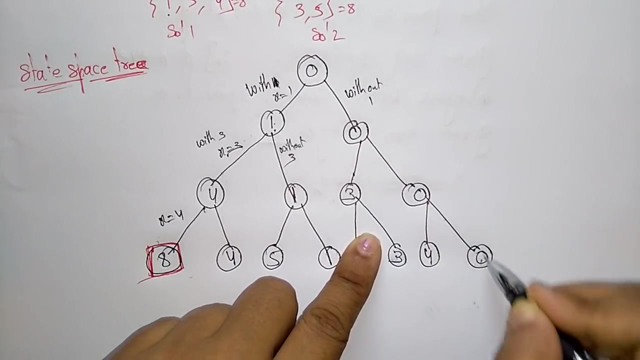 0 plus 3, 3 without 3, just copy 0. so this is: x is equal to 4 with 4. 4 plus 3, 7 without 4, just copy whatever the element that is there and here with 4, just 0 plus 4. 4 without 4, just copy 0. 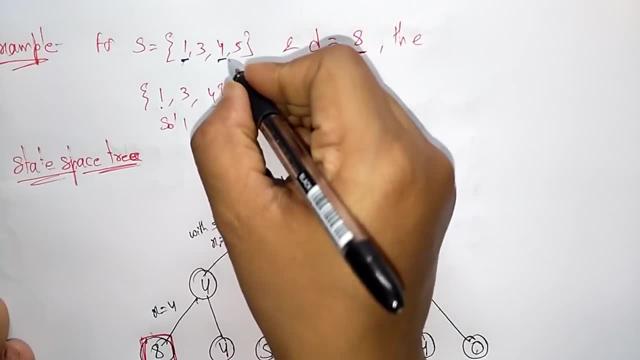 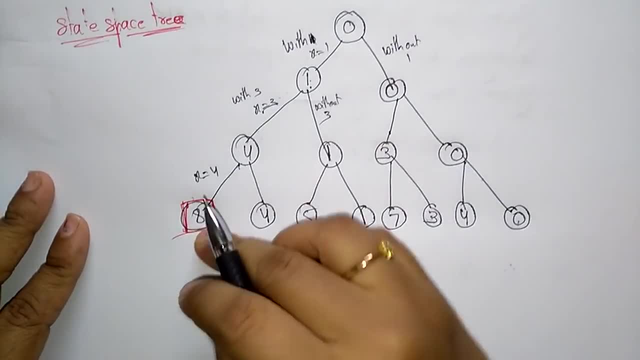 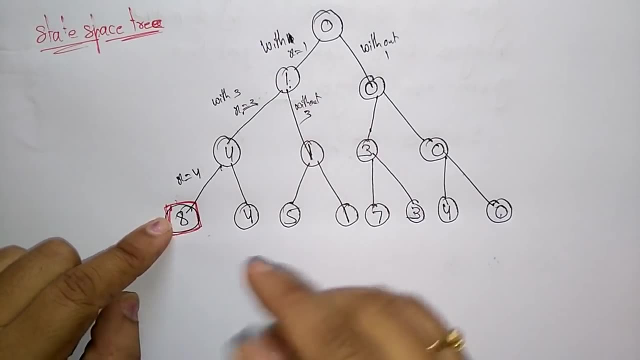 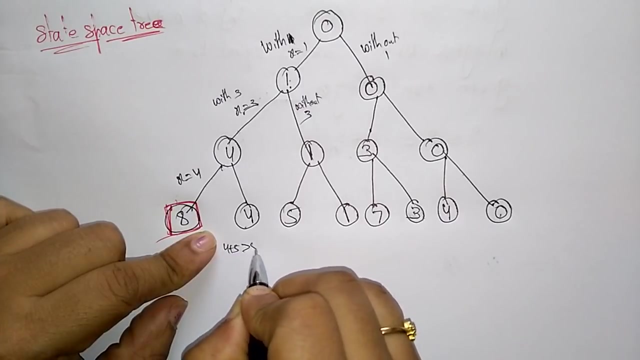 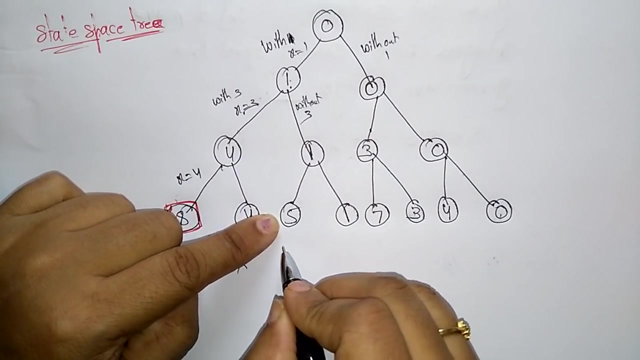 then last element in the set is 5. so here i got already. i got the solution, so no need to add elements to this leaf node. okay now. next coming to this: 4. so if, if i add 5 to this element, 4 plus 5 is greater than 8, so just skip this node. now coming to here. so if i add 5 here, 5 plus 5 is 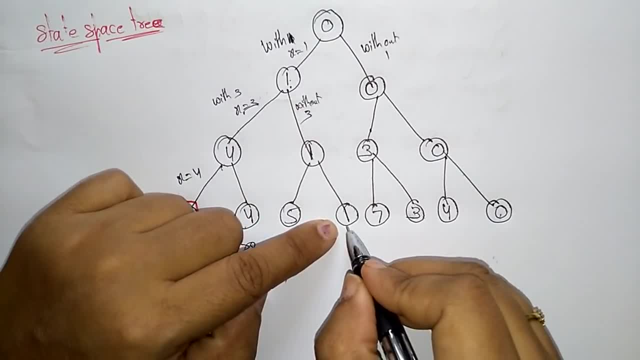 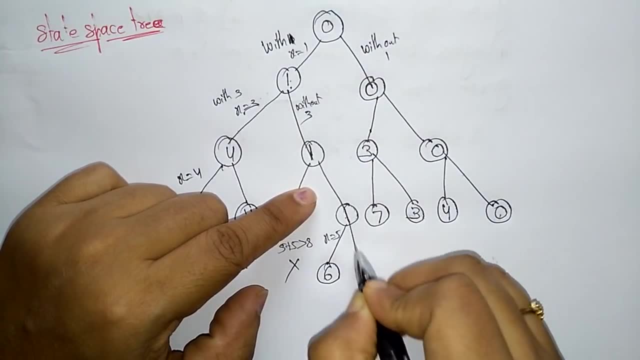 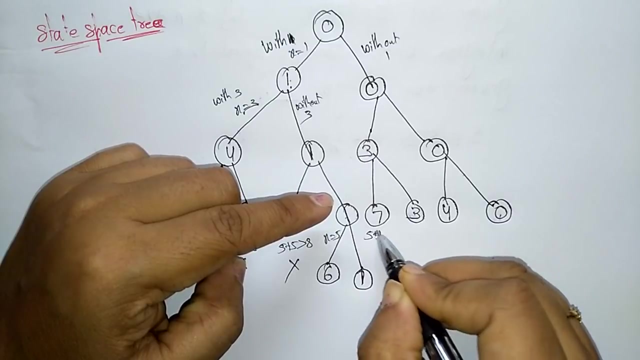 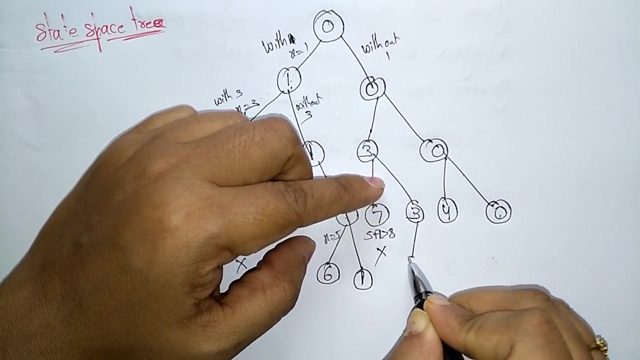 greater than 8, so just skip this node. now coming to here: now x is equal to 5, 5 plus 1, i'll get 6. and right side, just copy that one: 7. 5 plus 7 is greater than 8, so just skip this node. now coming to this: 5 plus 3: 8. i got the solution. 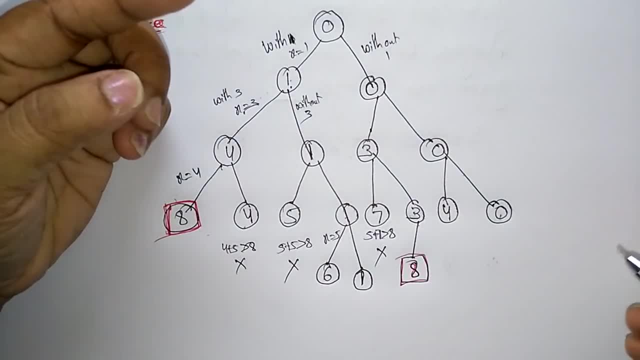 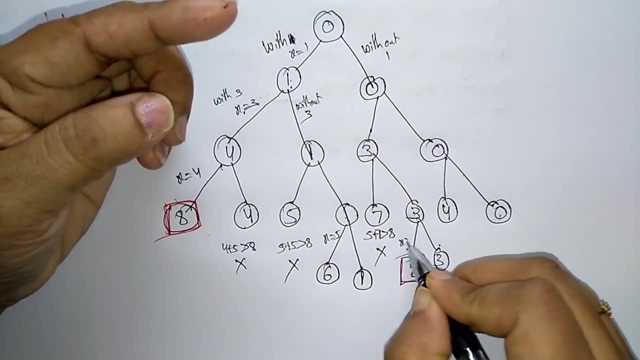 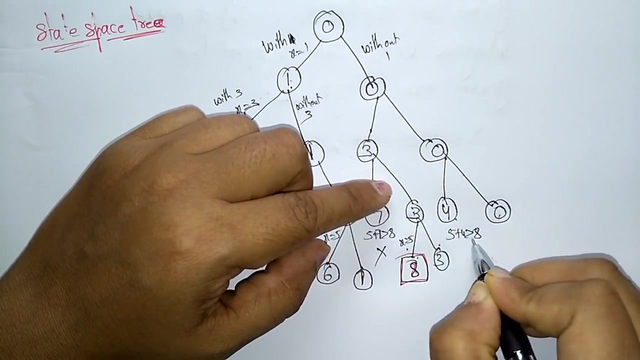 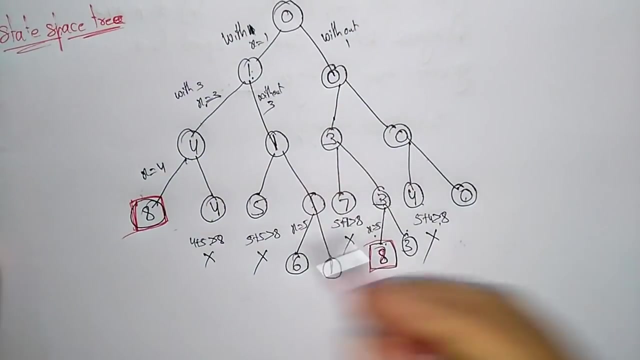 8. okay, and the right side is just copy that element with 5 without 5. so here x is equal to 5 with 5 without 5. now, coming to the 4, 5 plus 4 is greater than 8, so just ignore this, okay. so the total so, uh, what are the possible solutions that i get? 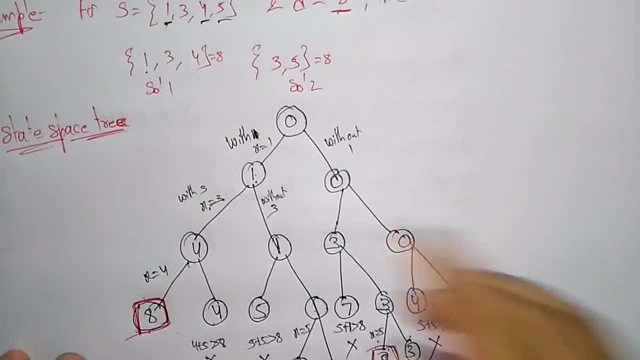 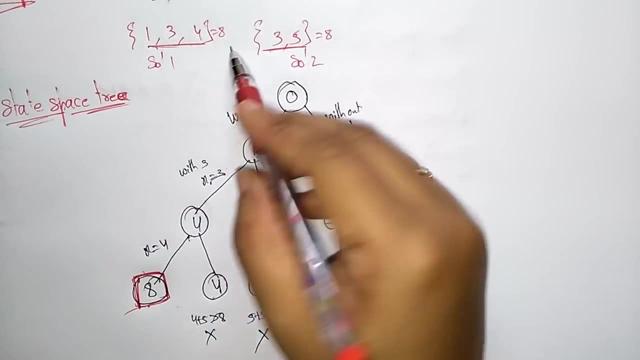 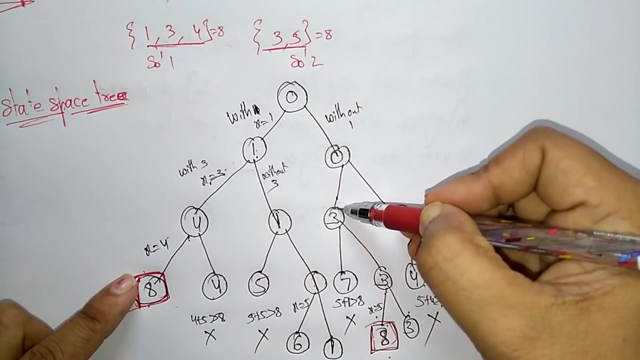 8 here and 8 here. okay, so i said i got, i will get two possible solutions. so 1 plus 3, 1, 3, 4. 1 plus 3 plus 4 is equal to 8 and here this is the 3, this 3 and 3 plus 5. here x is equal to 3. 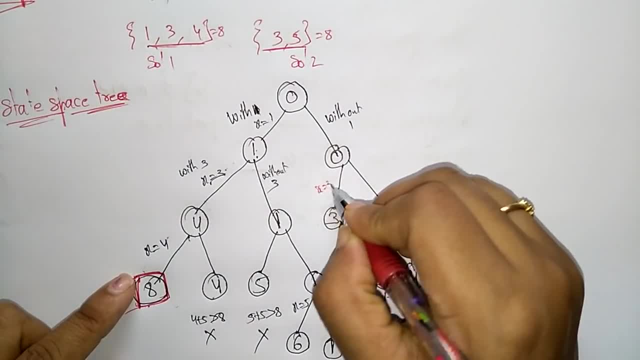 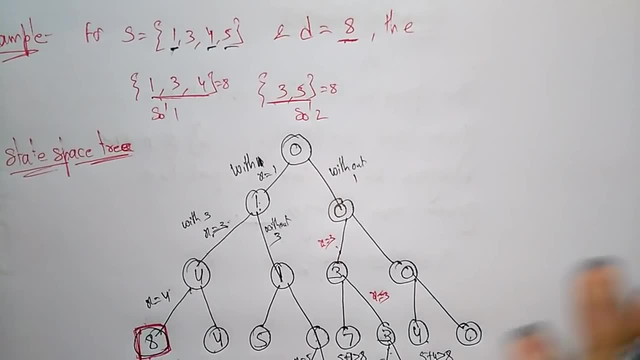 3 plus 5. you have to write here: x is equal to 3, 3 plus 5, 8. okay, so this is the sum of uh, sum of subset. by using uh. we are drawing by using the state space tree. thank you.